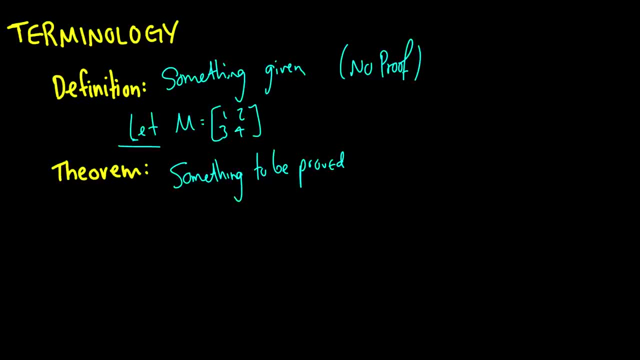 long definitions out while doing videos, I prefer doing them before. But a theorem is something to be proved and it usually results in these other sub proofs called corollaries, And what these are are these just happen to be little things that come about because the theorem is true. So if I have a theorem that says all, 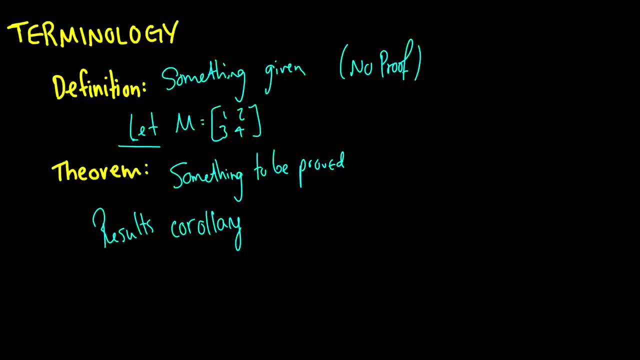 numbers are either odd or even the corollary is that any number divisible by 3, sorry, that's a really bad example- any number divisible by 2 is going to be even. So that's a little corollary kind of thing. Anyways, terminology is boring. 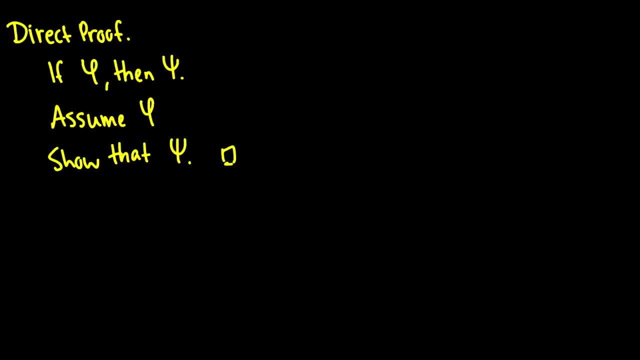 that's not why you're here. Let's get to the direct proof, and I'm using propositional logic because it is a very good way to explain how proofs are done. So in a direct proof we have a statement that says: if phi, then psi, and 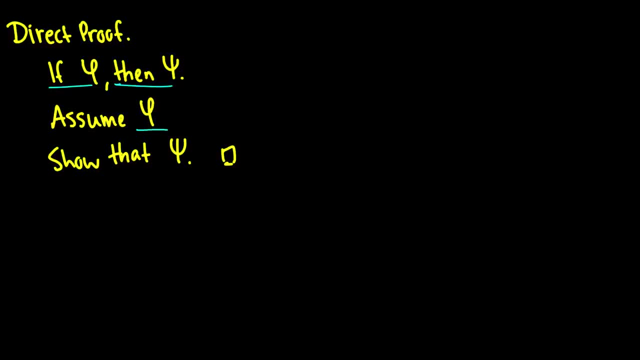 what we do here is we assume phi and we have to show that psi. So, for instance, if I say, well, let's just jump straight to the actual question, I wrote down: if x is odd, then x squared is odd. So first of all, 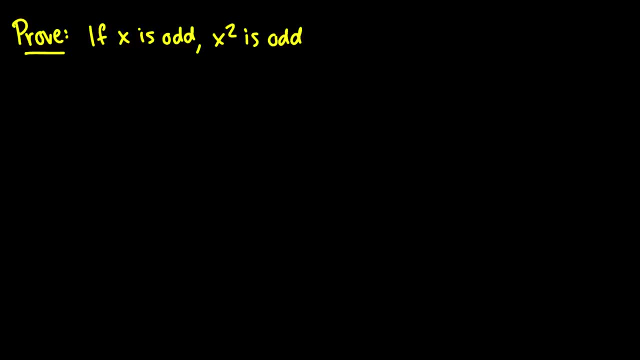 we're making an if-then statement. so to prove that it's true, well we say okay. well, let's just assume x is odd. Now, something about odd numbers is that any odd number can be written in the form 2n plus 1.. So now we have to prove that x, squared, is odd. Okay, 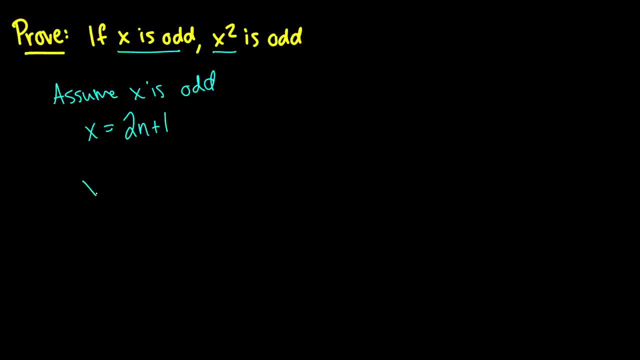 well, that shouldn't be too bad. Let's square both sides of this equation, so x squared is going to be the same thing as 2n plus 1 squared, which, if we factor this out, it is going to be 4n squared. 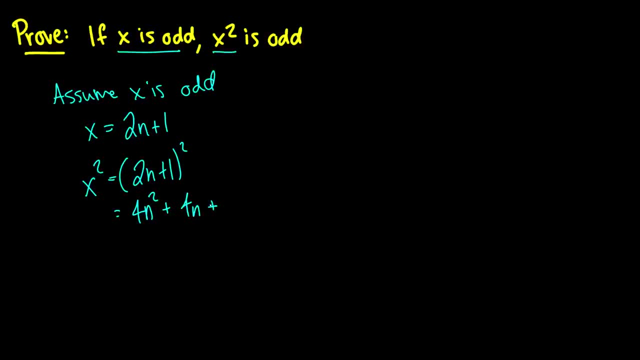 plus 4n plus 1.. Okay, so that's not too bad. So what we can see here is that we've actually proven that x squared is also odd, because we have- well, we know that 2n plus 1 is odd, so we could reduce it to 2n plus 1.. I'm not going to go that. 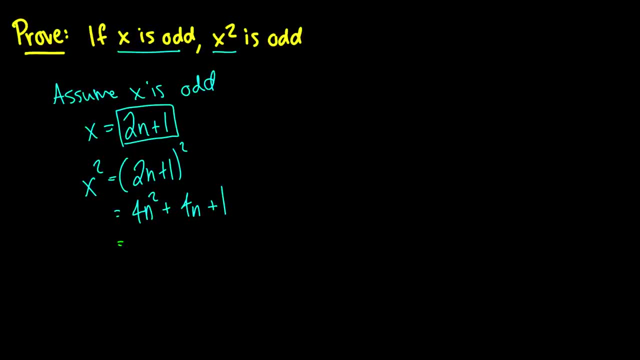 far. but I am going to say we can factor out a 2 and an n from the first two, so we get 2n plus 2, and then we get 1 out there, which really is, if you see this, this is 2n plus 1,. 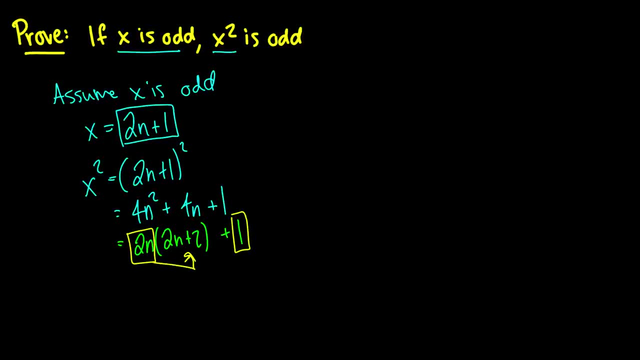 it just happens that the n has to be multiplied by an even number, which is 2n plus 2.. So we have actually proven that if x is odd, then x squared is odd. So that is a direct proof. It is a direct proof because we're assuming the antecedent is true, So I will repeat this again. 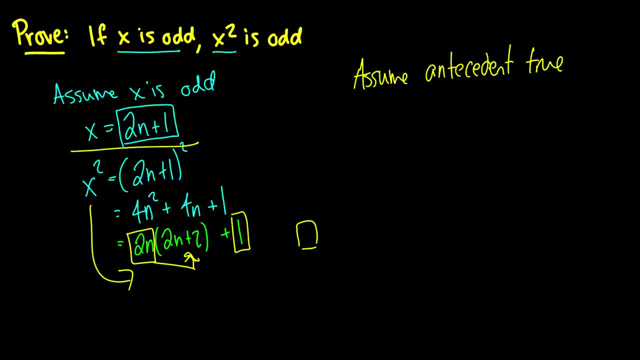 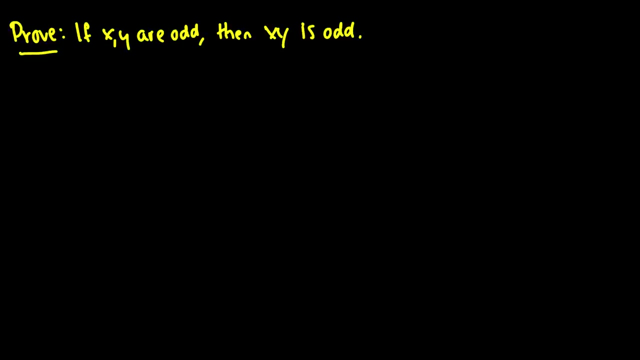 You assume the antecedent is true and then you prove the conclusion or the consequence, depending on vocabulary you wish to use, And that is a direct proof. I'm wondering if I have. oh yes, of course I have one more. There is a little section of direct proofs that I 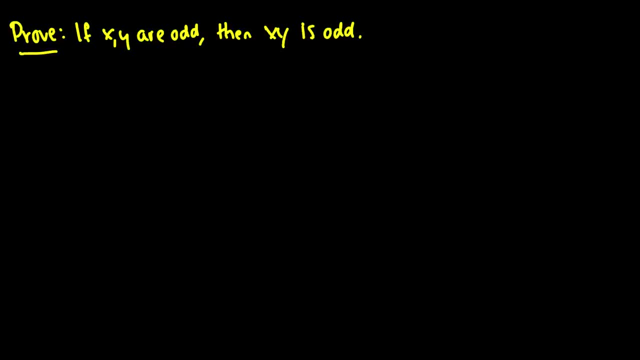 should cover now. I guess it's better to cover it now than later. but if we say if are odd, then are odd, Well, this isn't exactly crucial for this example. but if we were to say x or y, then we'd have to do a proof by case. 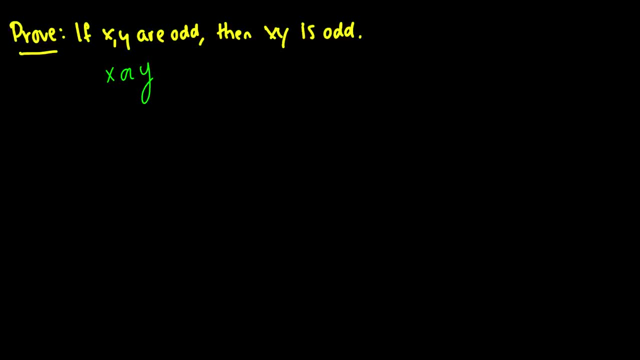 which is a little bit different. We have to take different cases where, okay, just x is odd and just y is odd, and then both are odd. We'd have to do that, but luckily for this, we're saying that both are odd, So we're going to let x be equal. 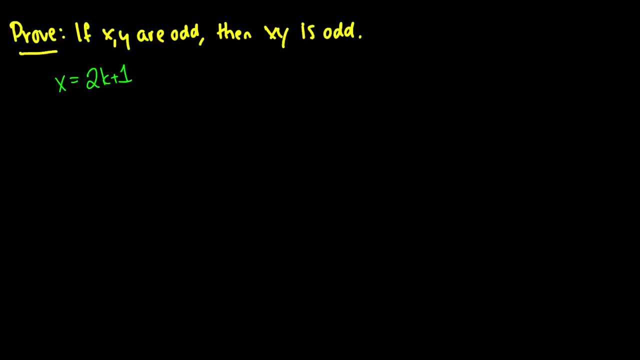 to 2k plus 1, and we're going to let y equal 2j plus 1.. So then x times y is going to be 2k plus 1 times 2j plus 1, which then, when we factor this out, we're going to get 4kj plus 2k plus 2j plus 1..